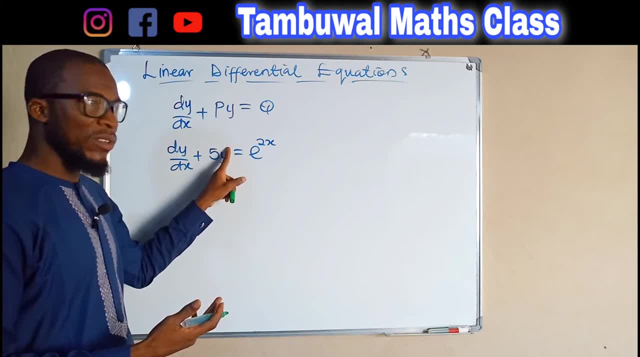 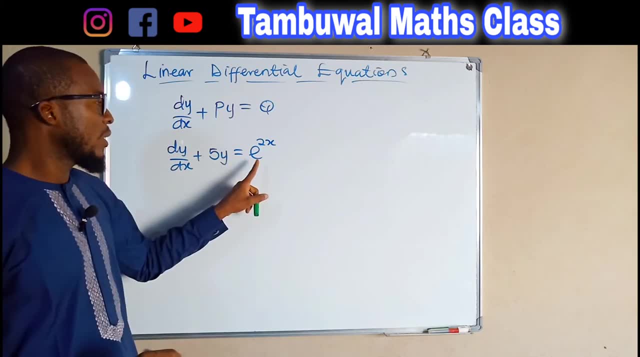 And we have 5y. here y is to the first degree. In a linear differential equation, y can never take any power apart from 1.. We have e to the 2x, where 2x is a function of x. 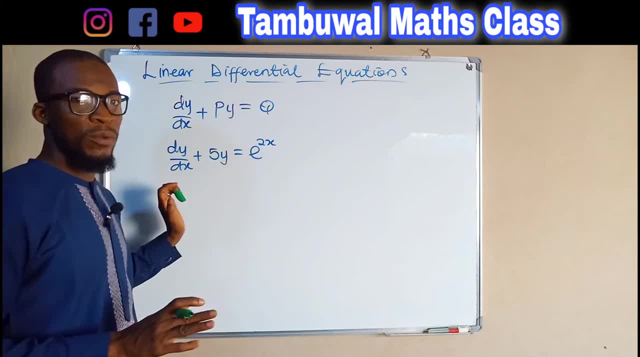 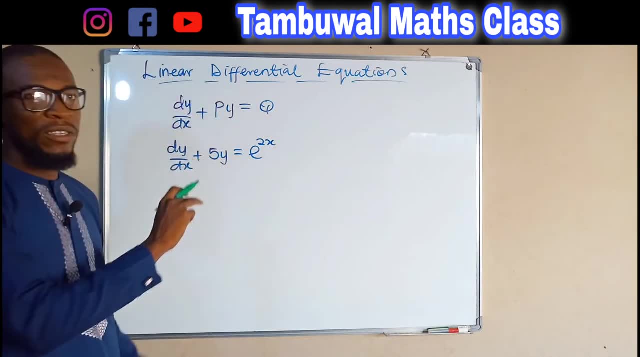 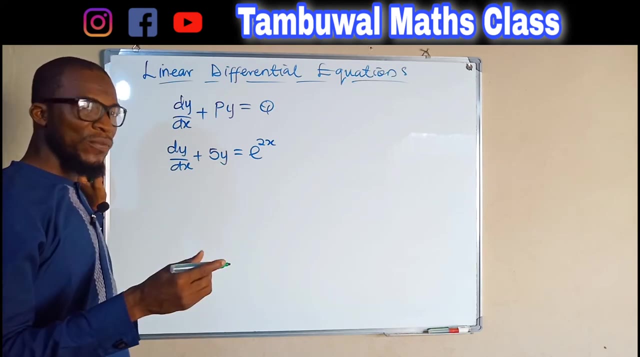 Suppose it is a function of y, we say it is a non-linear differential equation, And again, none of the methods we applied initially can be used in finding the solution for this form of differential equation. Hence we are going to obtain a particular factor, which we call integrating factor. 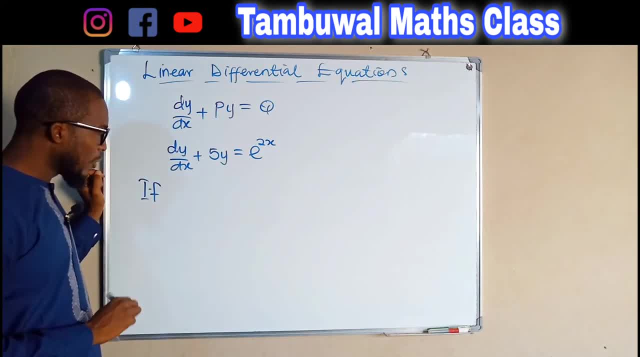 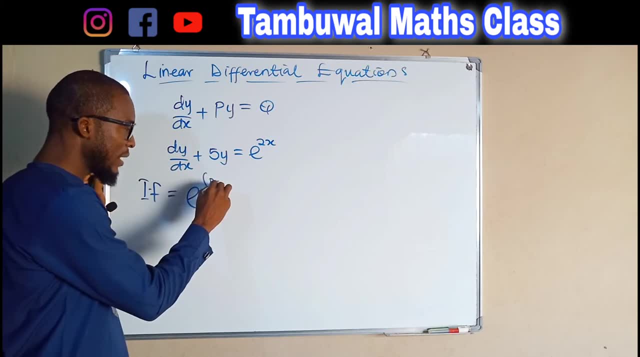 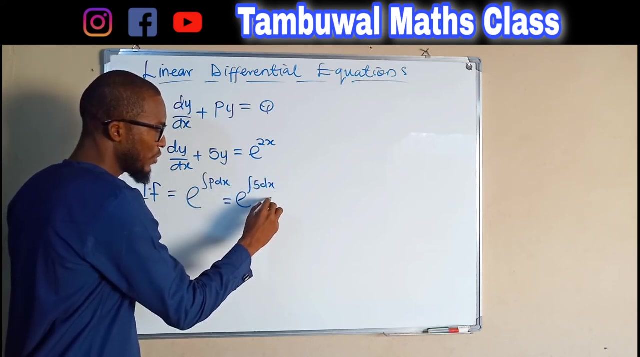 Integrating factor. And to obtain that integrating factor, we are going to take e to the integral of p, dx. And you know, p is the coefficient of y, which we have here as 5.. So this is equal to e to the integral of 5, dx, which is equal to e to the 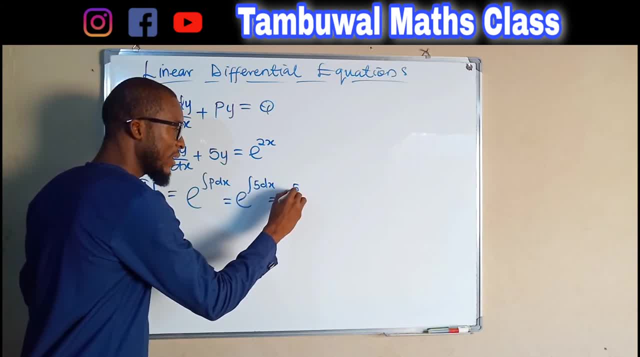 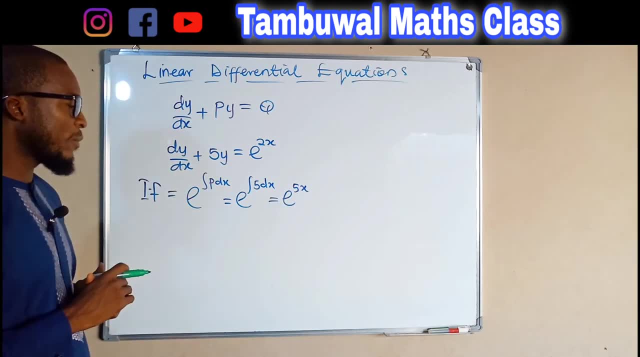 If you take the integral of 5 dx, you are going to get 5x. Hence, e to the 5x is our integrating factor for this differential equation. What we are going to do, we are going to multiply each of these terms by this integrating factor. 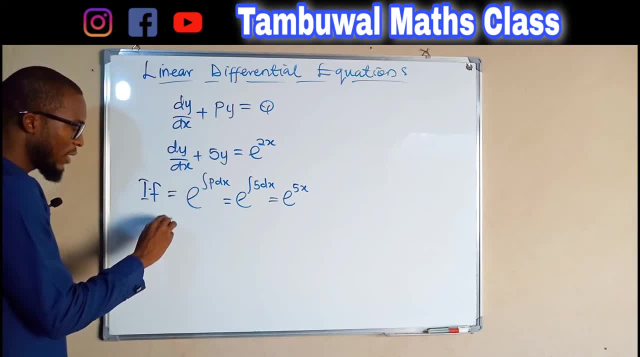 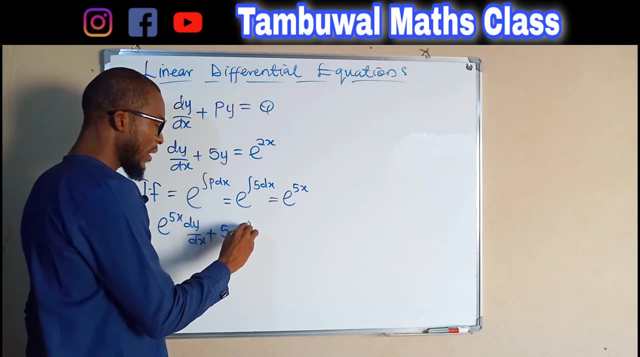 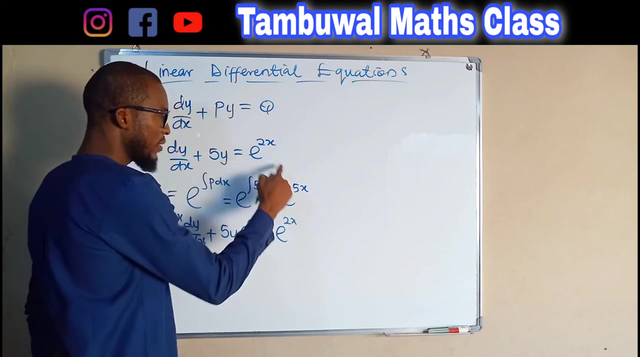 So the first term, we have e to the 5x, dy over dx. plus We have 5y e to the 5x. This is equal to e to the 2x, which is this. Then multiply it by our integrating factor, which is e to the 5x. 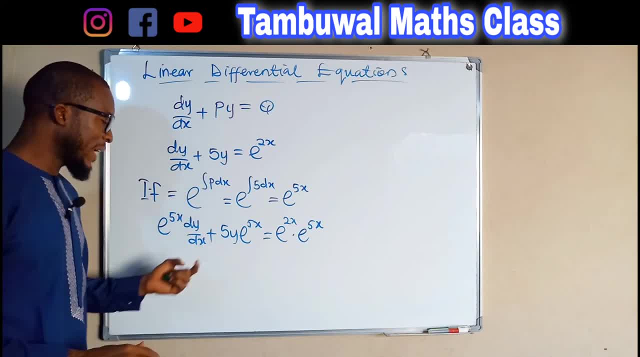 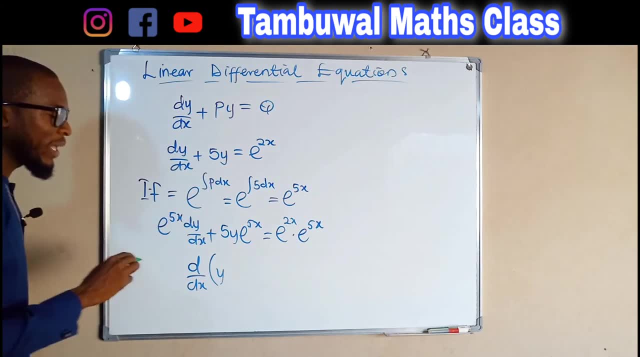 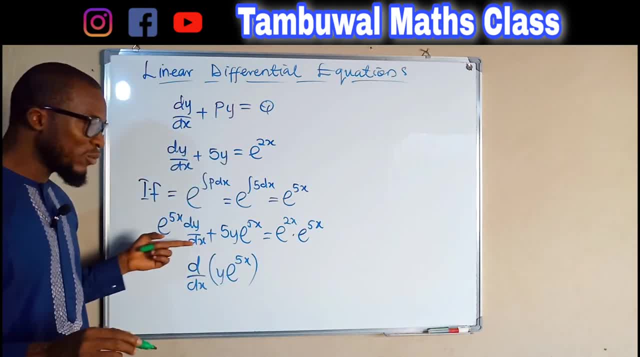 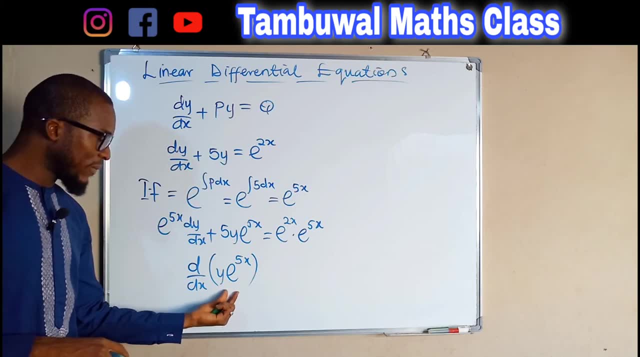 If you differentiate this, you are going to get these terms, these two terms, exactly. Hence we can write them in this form. If you want to find out, you can take the derivative of these terms. using product rule, You keep y constant. 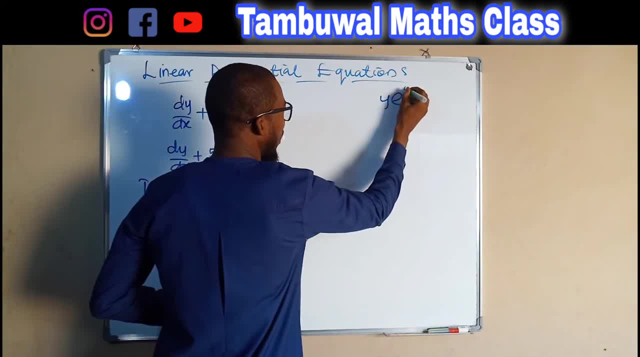 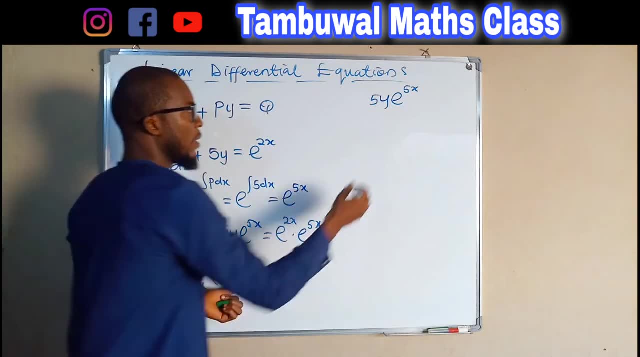 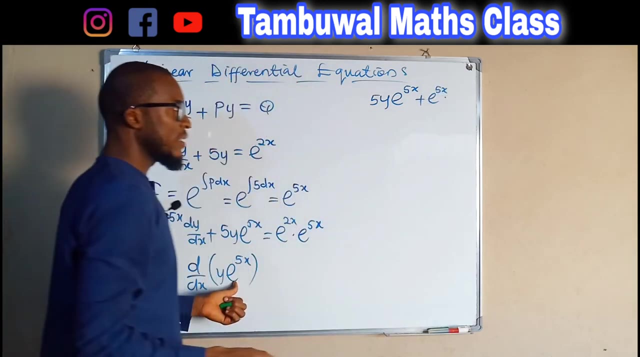 You take the derivative of the second, which is e to the 5x, multiplied by the derivative of the power y, which is going to make it 5 plus. now you keep the second one constant, e to the 5x. then you take the. 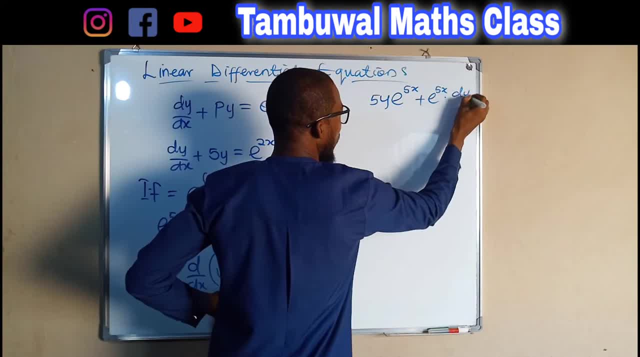 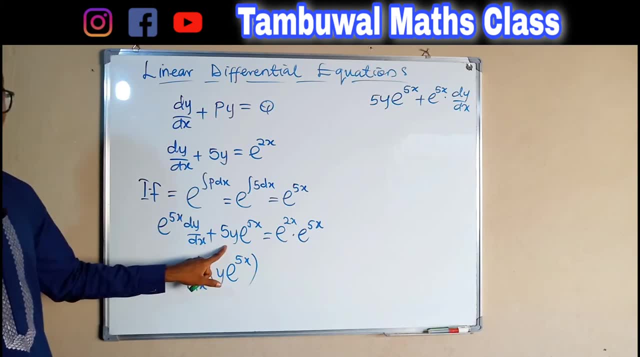 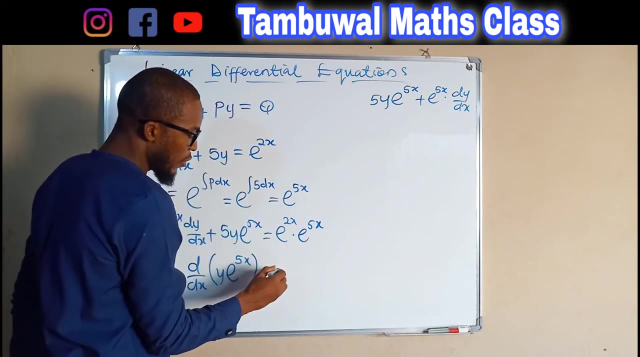 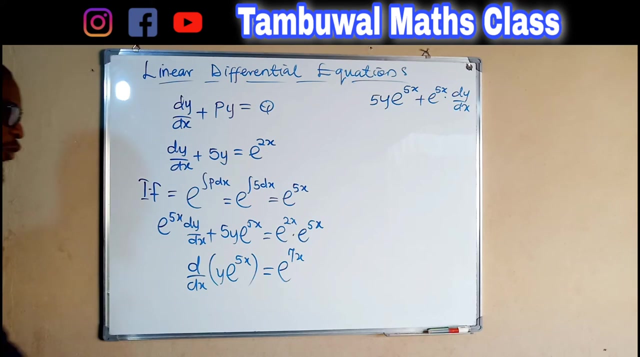 derivative of the first, which is dy over dx. If you look at these two terms, they are exactly the same with these ones. hence we can write them in this form. and to the right hand side, using lots of indices, you can take one base and add the powers together: 7x. Now we can go ahead and 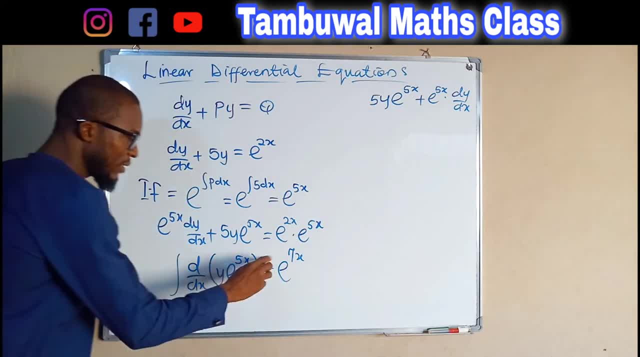 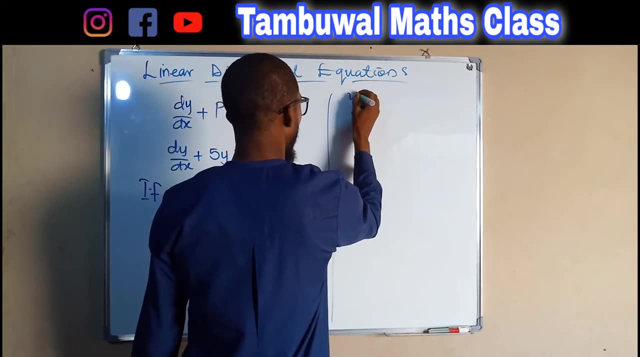 integrate both sides. Integrate the left hand side, Integrate the right hand side. with respect to x. If you integrate the left hand side, you'll be left with only y exponential 5x, y exponential 5x, 5x. this is equal to. 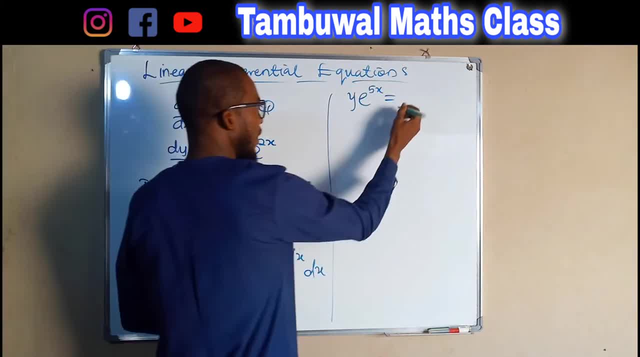 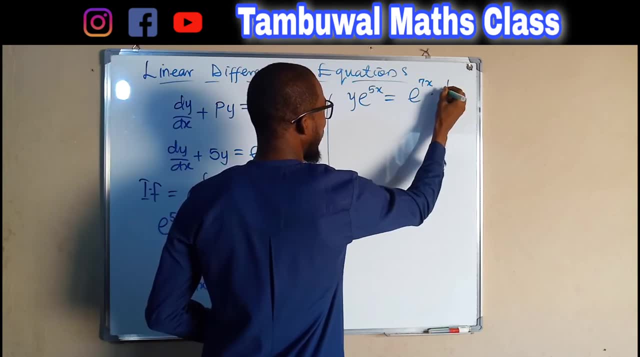 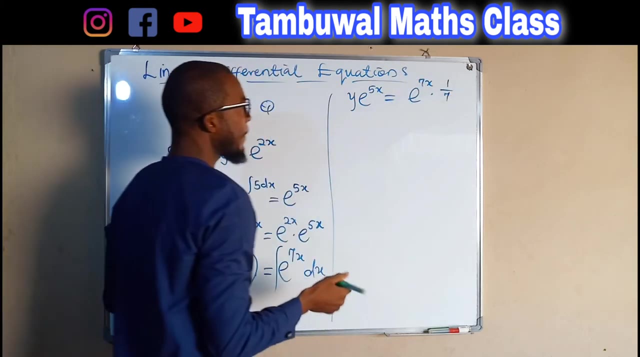 if you integrate this, you're going to obtain e to the 7x multiplied by 1 over the derivative of the power. if you differentiate 7x, you're going to obtain 7.. This is the same thing as y exponential 5x equals. 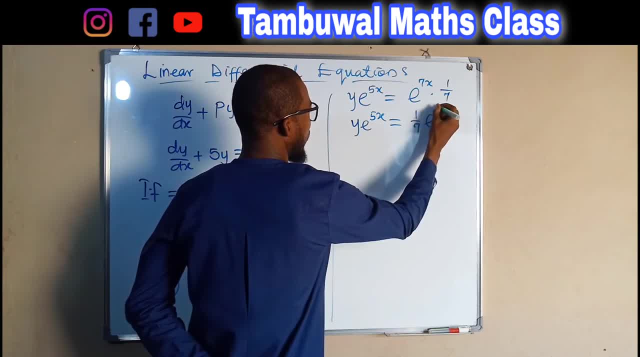 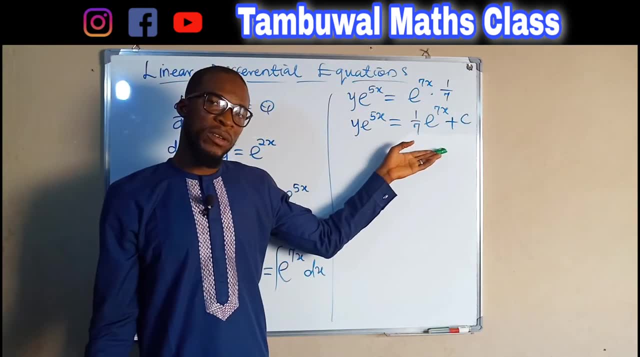 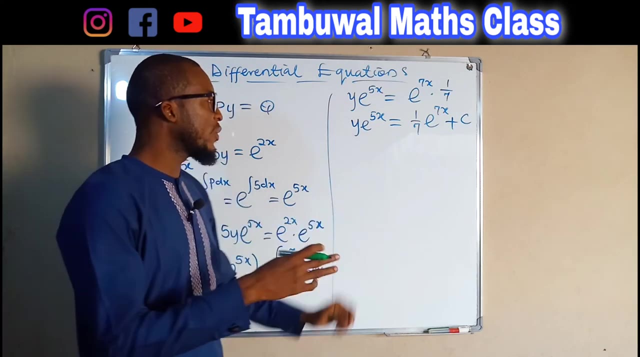 1 over 7, e to the 7x, e to the 7x, plus our constant of integration. hence you can leave your solution in this form and, if you like, you can divide both sides by e to 5x and other to have y alone. so we have y if you divide both sides by this, and this is equal to: 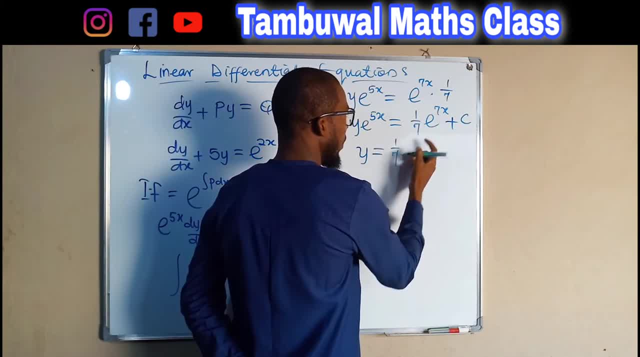 1 over 7, divided by e to the 5x, using lots of indices, 7 minus 5 is 2, so we will have y maximum and a, j is no more than e to 5x plus z, t, which other i we can pureете or we divide both. 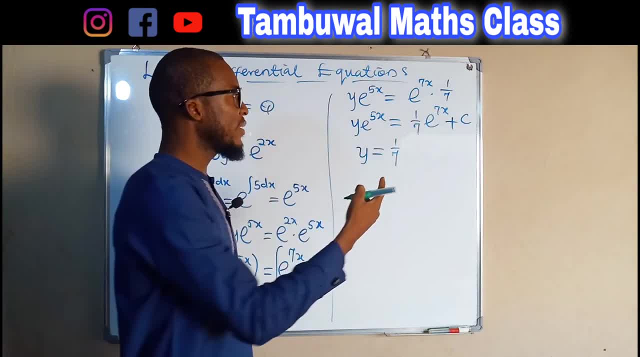 y alone, Y Alon diagram. and if you divide both sides by this, and this is equal to 1 over 7. e to the 7x divided is equal to 1 over 7, e to the 7x divided by e to the 5 x, using lots of indices, 7 minus 5 is 2. so by the fact of it, say we will take, is less. 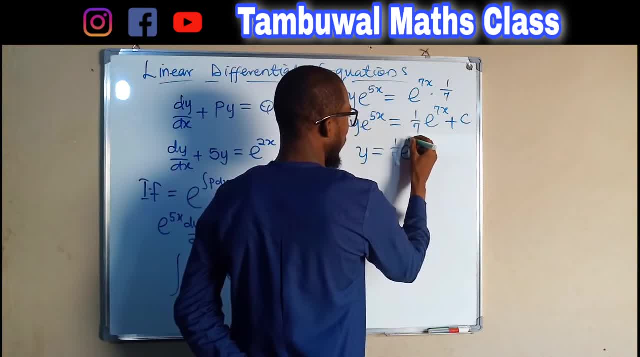 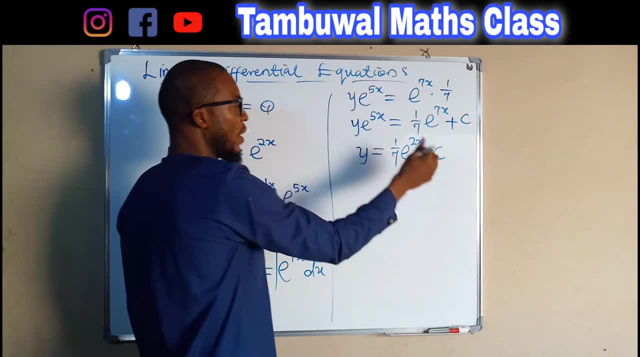 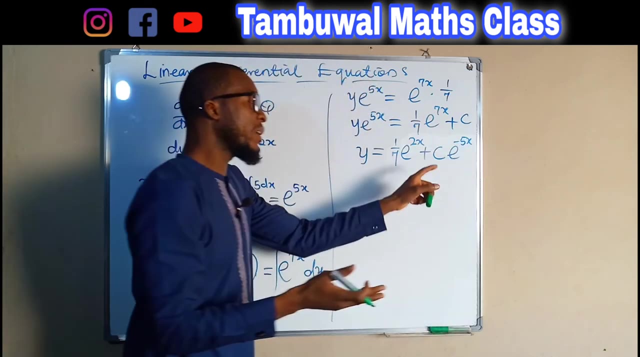 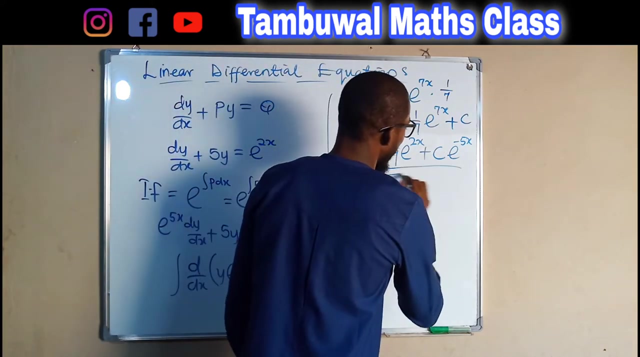 5 is 2, so we have exponential 2x, plus we have c. You can take the inverse of this power so that you can multiply c with e to the negative 5x. It is the same thing as dividing c with e to the 5x. Hence, this is the solution for this linear differential equation. So now, 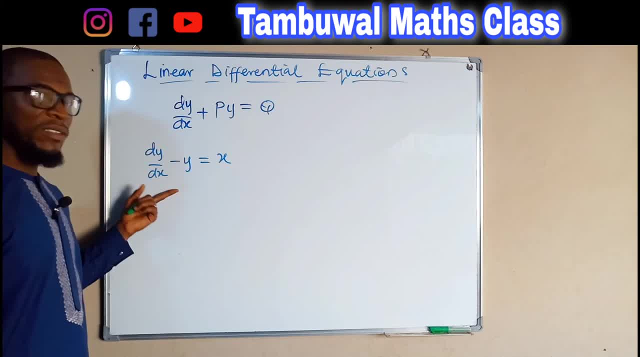 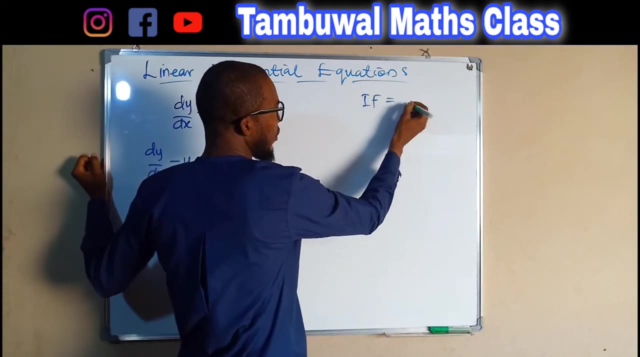 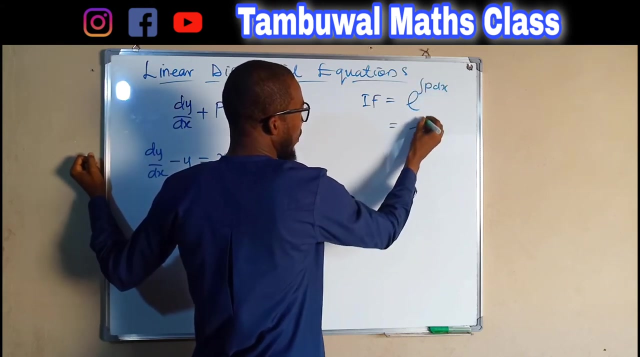 let us look on to the second problem. Now here is our next problem. We have dy over dx. minus y equals x. First thing we are going to find our integrating factor. Our integrating factor is always equal to e to the integral of p- dx. This is equal to e to the integral. 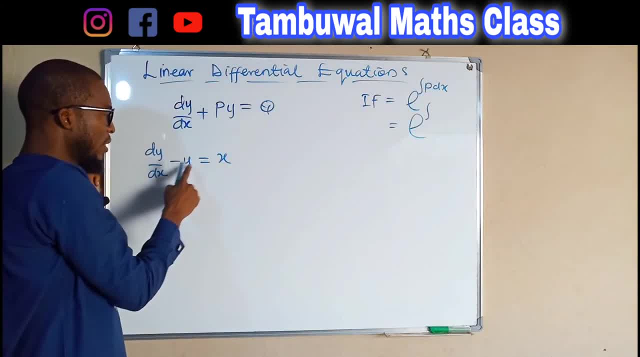 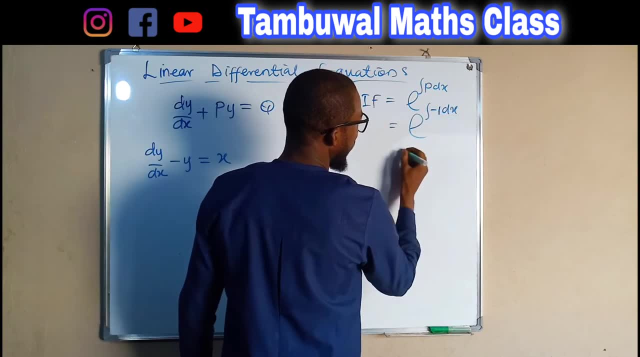 of our p, which is the coefficient of y, And we have the coefficient of y here to be equal to negative 1.. So we have negative 1 dx. This is equal to e, to the. if you take the integral of this, you are going to obtain: 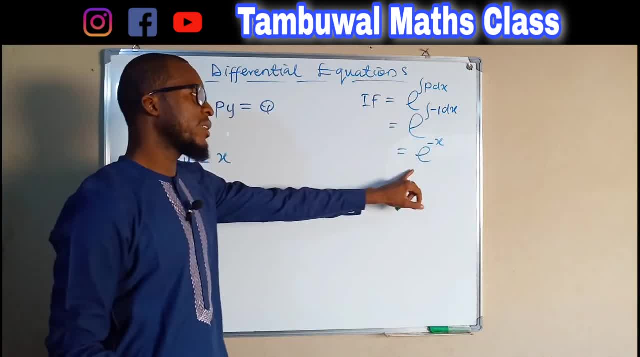 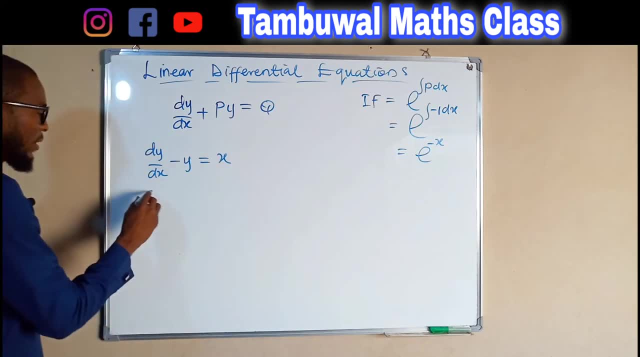 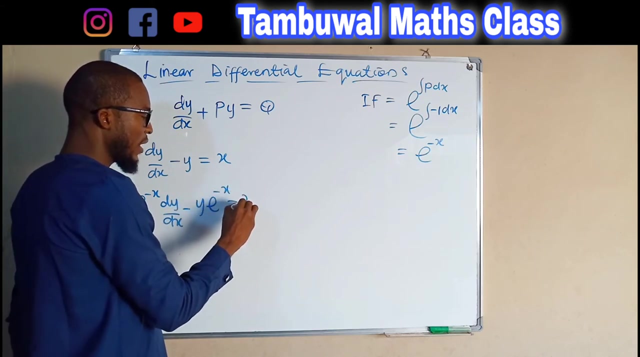 negative x And this is our integrating factor. We are going to multiply each of these terms by this integrating factor, The first one we have: e to the negative x, dy over dx plus y minus y. our integrating factor: e to the negative x. This is equal to x multiplied. 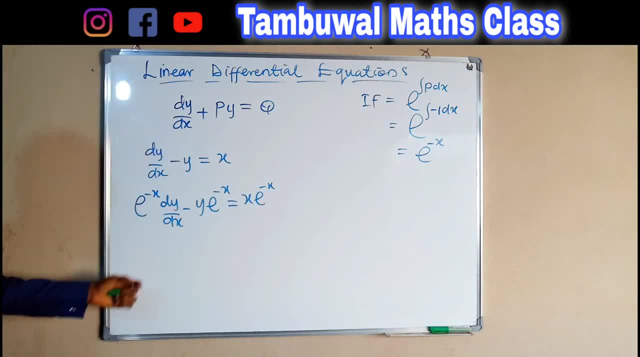 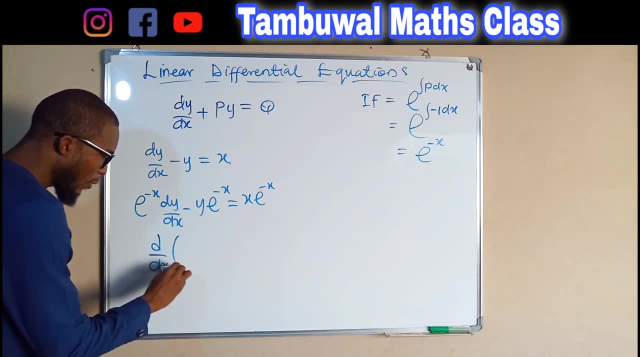 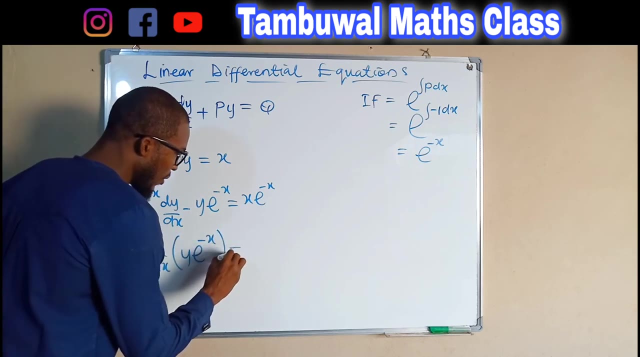 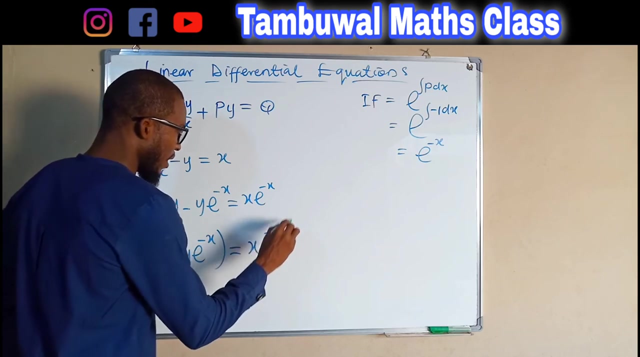 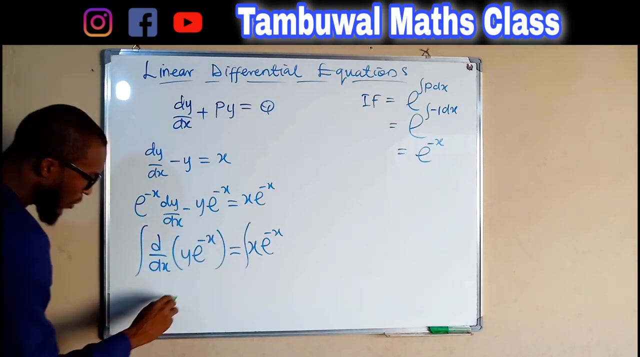 by e to the negative x. Remember I told you, the left hand side can always be expressed as dy over dx of y multiplied by the integrating factor which is e to the negative x, And we have to the right hand side x. This is the once. 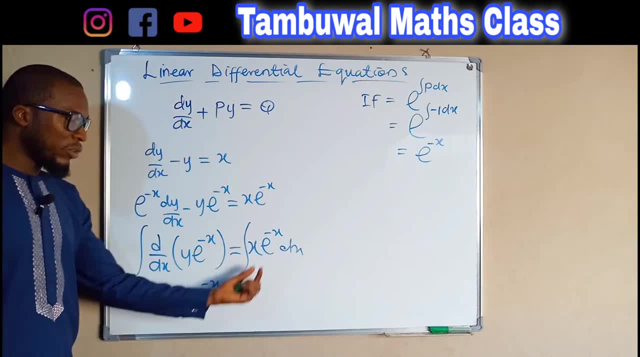 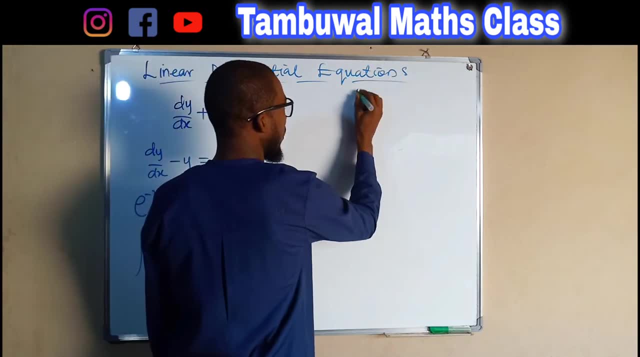 time the ñ direction equation showing that I take the25, I can leave in the next μ and w. I take the 25.. I speak mark, I grab a specificboom. I don't know how many times I just move. Ifmu concepts, trunk, ethnic paper. It is an expression. 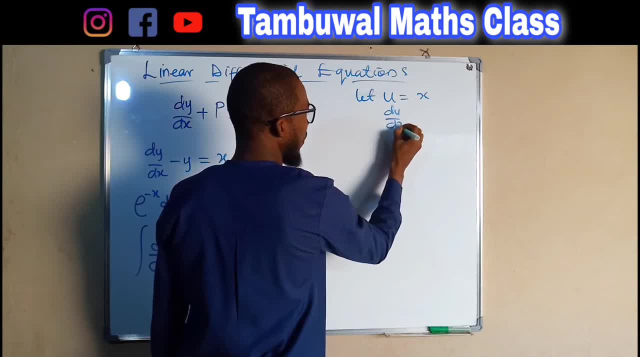 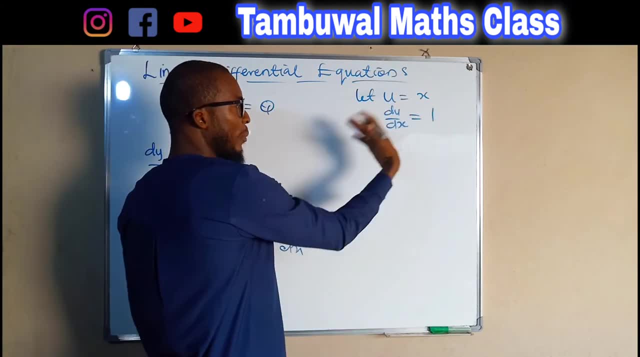 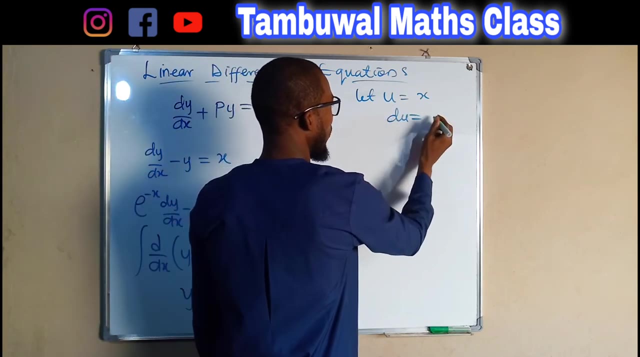 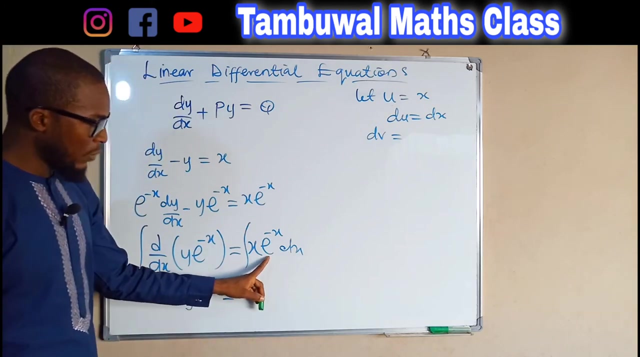 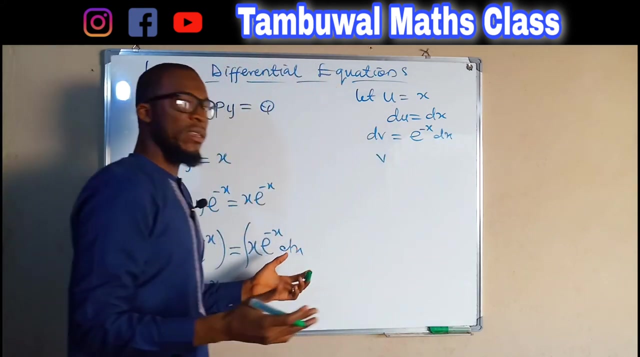 du over dx is equal to 1.. If you take the derivative of u with respect to x, we are going to obtain 1.. So by multiplying both sides by dx, we are going to obtain du equals dx. Then we take dv to be equal to the remaining term, which is exponential negative x, dx, V. by taking 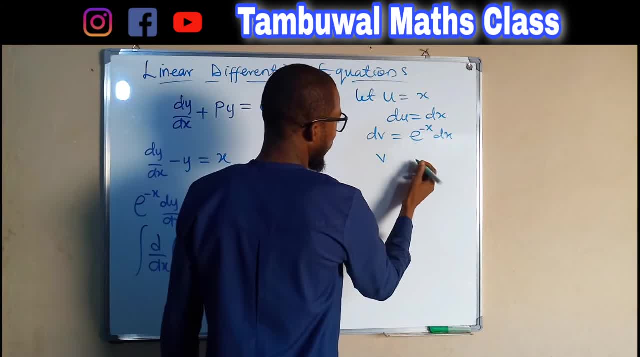 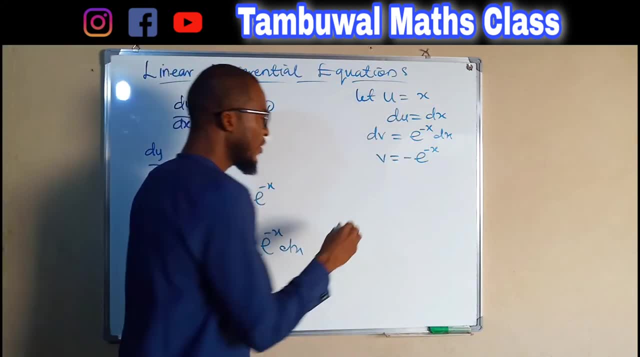 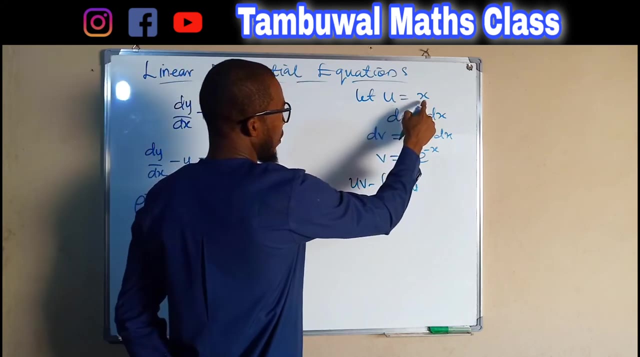 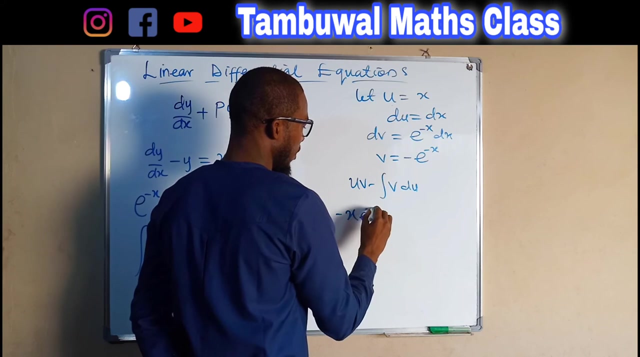 the integral of both sides. this is the same thing as negative, exponential, negative x. So we are going to substitute this into uv minus the integral of v, du. Our u is x, Our v is exponential, exponential e to the negative x, But we have our negative at the back. 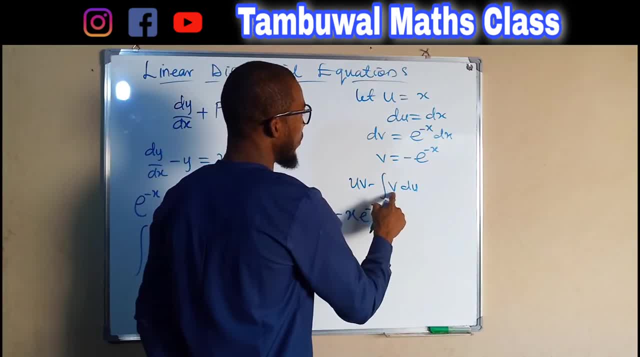 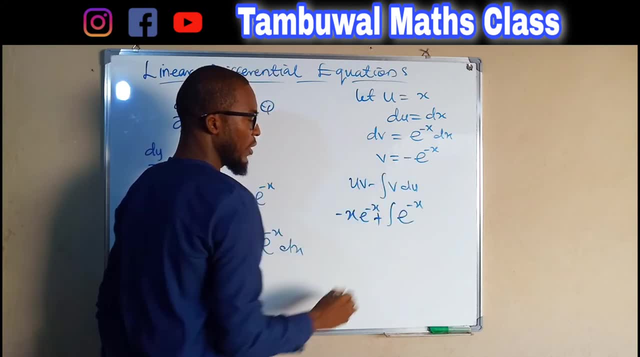 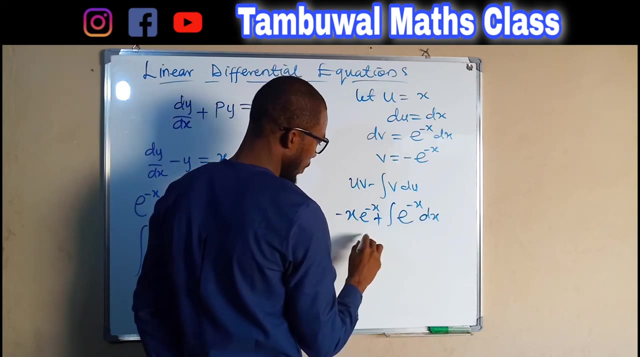 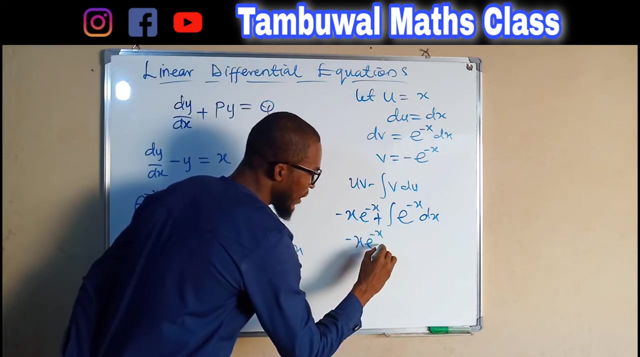 minus the integral of v. What is v? We have negative e to the negative x, So this negative can come out to make this positive. And we have du to be equal to dx Minus x, exponential Minus x. exponential, negative x. If you take the integral of this, you are going to obtain negative. 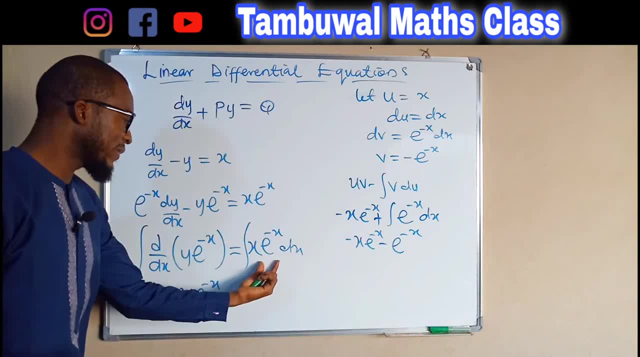 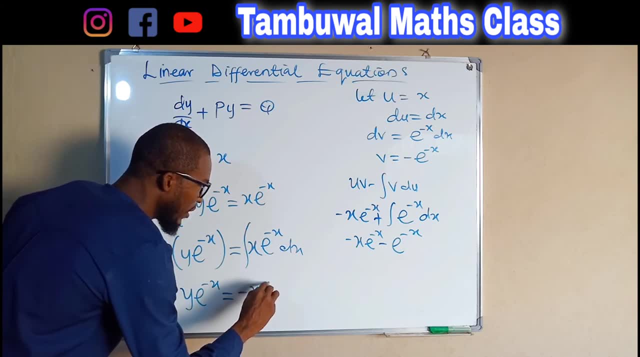 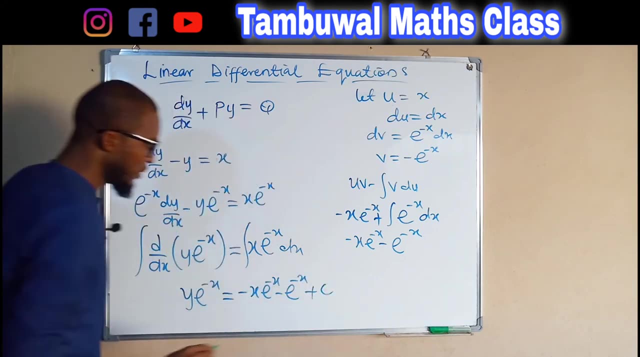 e to the negative x. Hence we can substitute this with this: This is equal to minus x, e to the negative x, minus e to the negative x, plus the constant of integration. We can as well divide both sides by e to the negative x. 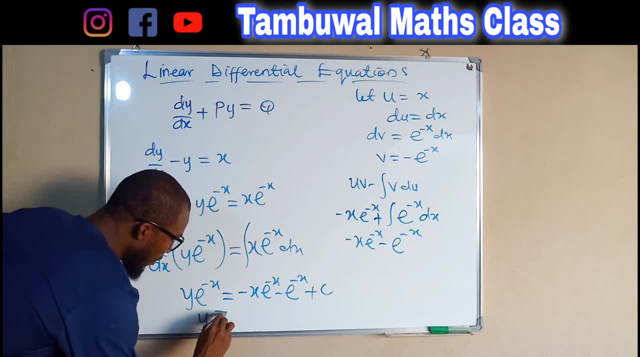 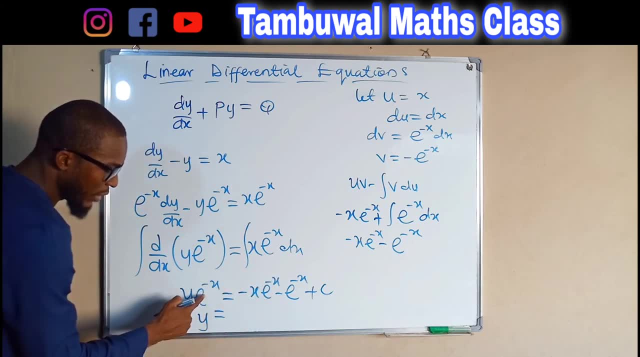 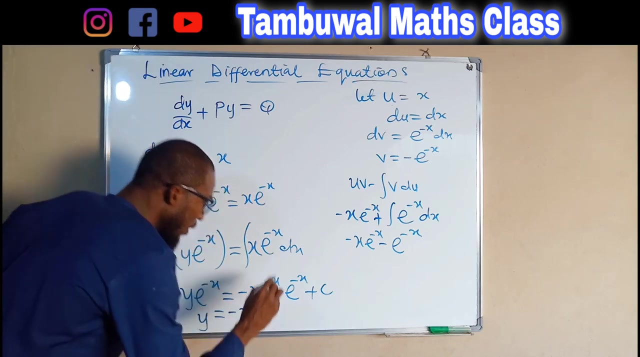 Leaving y here. and this is equal to If you divide this term by this, because e to the negative x will cancel e to the negative x, Leaving only negative x here Minus, We have e to the negative x, We have e to the negative x. They will cancel Having one Plus Constant. 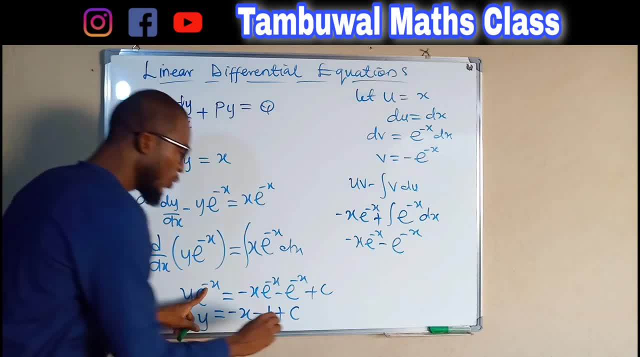 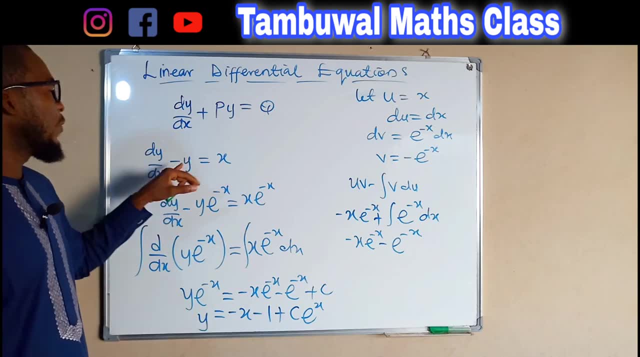 You can take the inverse of this, so that they will multiply as e to the x, And hence this is the solution for this differential equation, And this is all I have for you today. Thank you for watching. Do have a nice day.